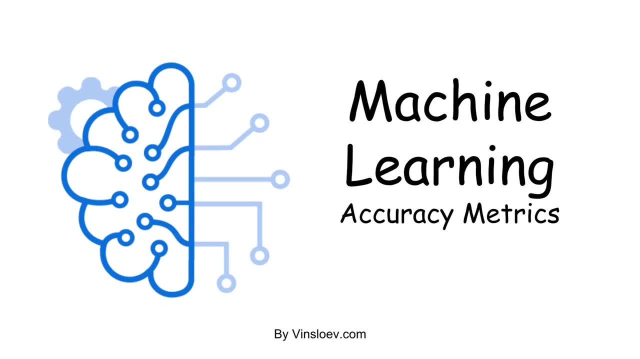 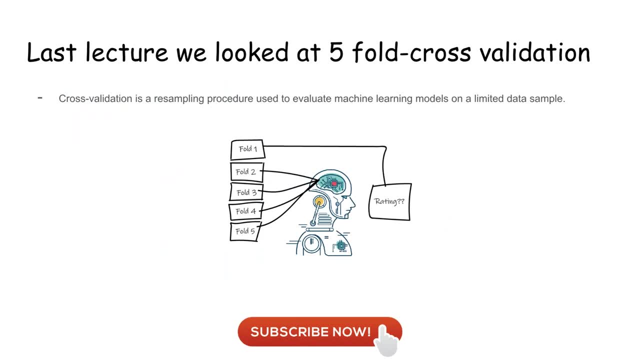 Hello and welcome to Winslow Academy. In this lecture we will look at machine learning and how we can measure accuracy by using accuracy matrix. So in the last lecture, which were part 7 in this tutorial guide of basic machine learning in Python, we looked at how we could use 5-fold crest validation to split up our training. 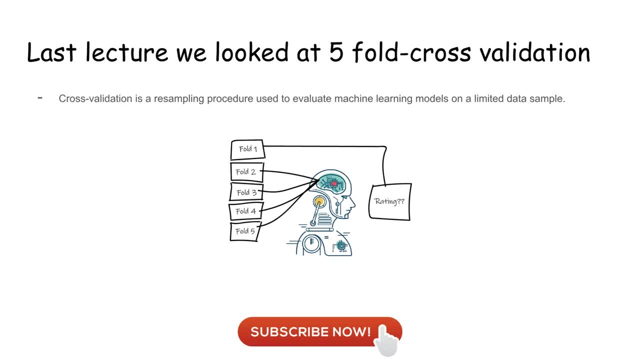 set and hide some of the values in order to use these as test values to measure how accurate our algorithm were. If you are interested in learning how to use this 5-fold cross-validation method, then please go to the channel and find part 7 of this tutorial, and then you can rewatch it all. 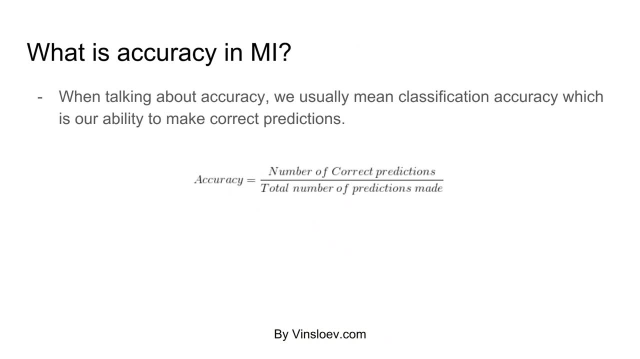 But now let's continue with the accuracy matrix. So what is accuracy in machine learning? So when talking about accuracy, we usually mean classification accuracy, which is our ability to make correct predictions. So our overall goal when predicting something and using machine learning algorithms is to 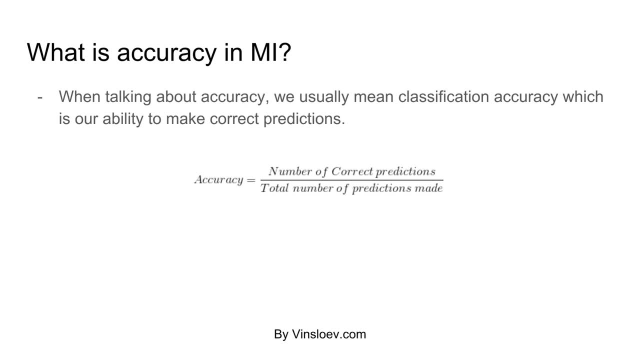 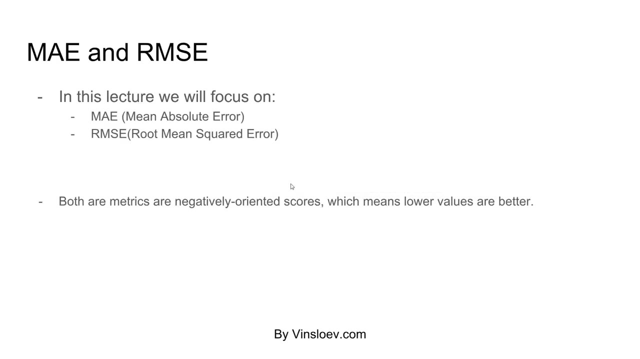 do so is to have as accurate a result as possible. So the accuracy can be measured by saying the number of correct predictions divided by the total number of predictions made. And the way that we are going to measure this is by using two of the most famous matrix. 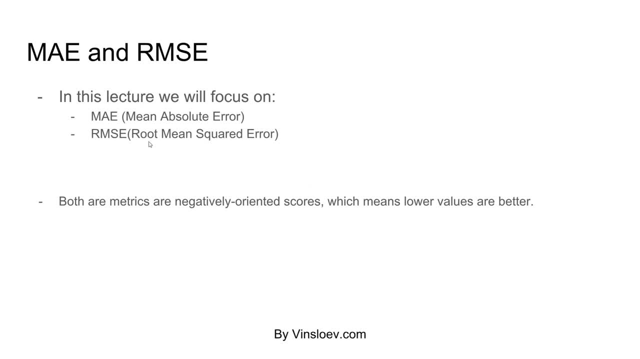 of doing so. the mean absolute error and the root mean squared error, So both of these are negatively oriented scores, meaning that the closer you get to zero, the more accurate your algorithm is. So, basically, we want, in the ultimate scenario, to hit a score of zero, because then our algorithm 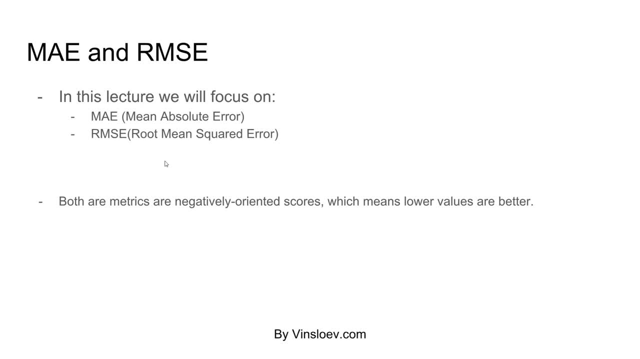 is capable of predicting exactly the same score that real users have given, And then we most likely have one of the best algorithms trained in the world, if we can do so for all examples. So that is, of course, a dream scenario, but that is what we are aiming for. 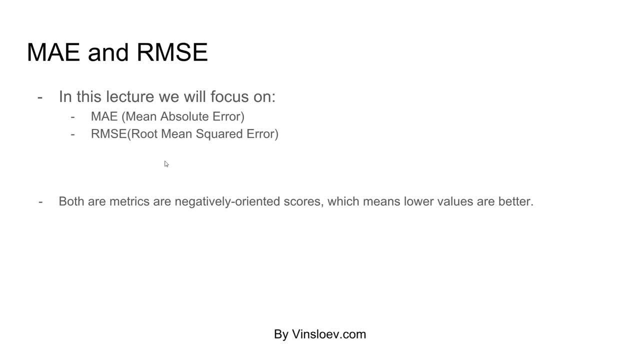 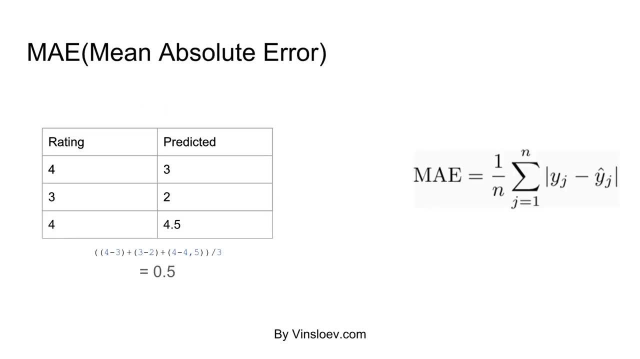 And now we will learn how we can calculate these scores based on some numbers that we have. So if we start by the mean absolute error, we have the formula right here And, as you see, we will take the sum of all our ratings and predictions, minus them into. 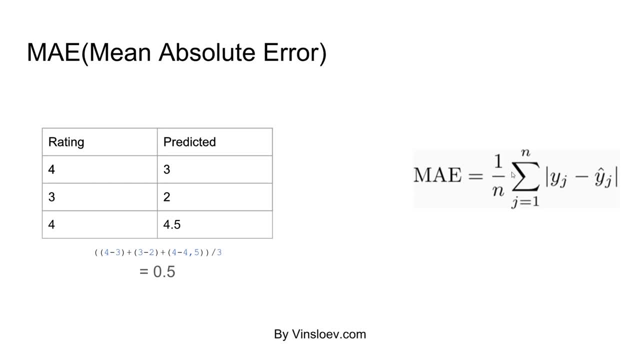 absolute error sets and then we will sum them together and divide by the overall number of ratings or occurrences. So If we take the yj right here, then that is for the first value, it is 4 minus 3.. Then we take the next value, which is 3 minus 2, and so on. 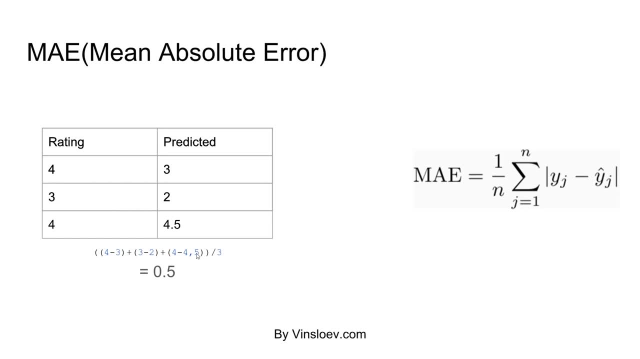 And, as you see right here, this is illustrated in a more calculation-friendly way. We take 4 minus 3, calculate the value of that plus 3 minus 2, calculate the result of that And add it together with 4 minus 4.5. 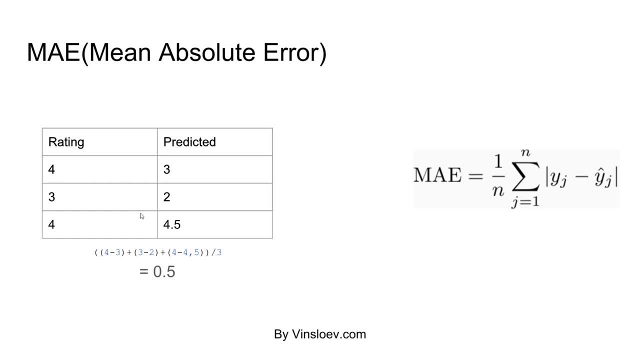 And then we take the summation of all these and divide it by 3, because we have three set values right here, And the end result of this is MAE score of 0.5,, meaning that our algorithm has a mean absolute error of 0.5,, telling us that we have a mean of around 0.5 of the real values. 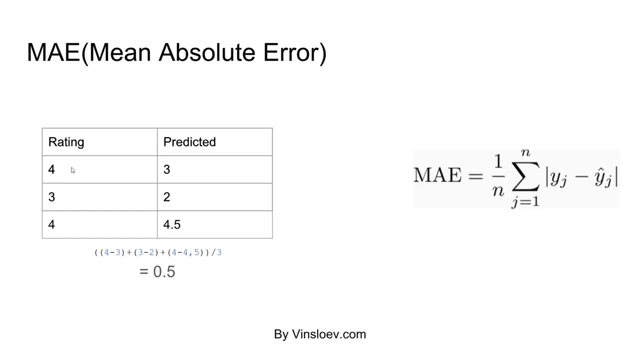 in overall, But again, this is only a data set of three items, so this is not saying that much about our algorithm, but this is the way that we are going to calculate this, and this can be used on a data set where you have 10,000 or 100,000 results and then you really start. 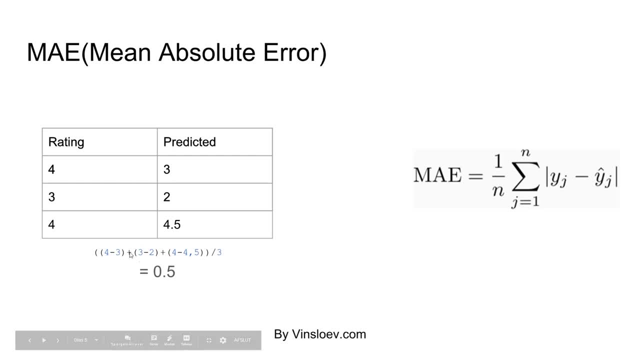 to see some information from this MAE and you can actually use it for something, because then, when you have started to manipulate the parameters of your Machine Learning algorithm, then you can see whether this is true. this score goes up, meaning that you get a worse result, or it goes down, meaning that 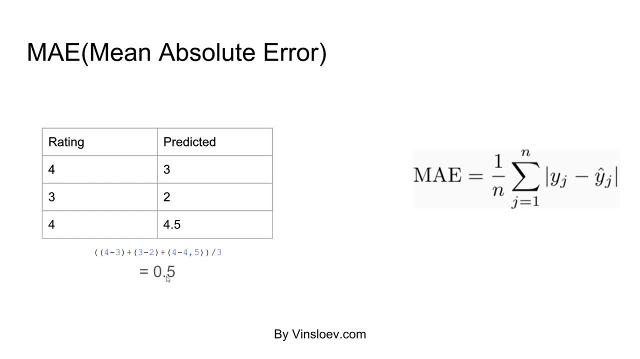 you are doing something right and the algorithm is actually getting better at predicting these values. The other score is the root mean squared error, which penalizes a lot more on the larger errors. So if we take the exact same values right here and then we have the formula right. 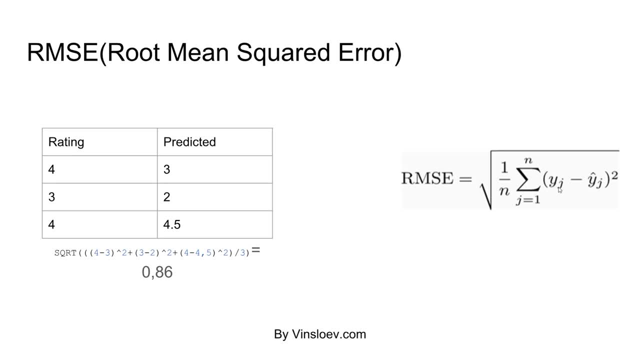 here it is the same again where we take the yj. here is 4 minus 3, which is the predicted value. Then we take that value and then we sum these together as we see right here: So 4 minus 3 to the power of 2,, plus 3 minus 2 to the power of 2, and so on, And then again: